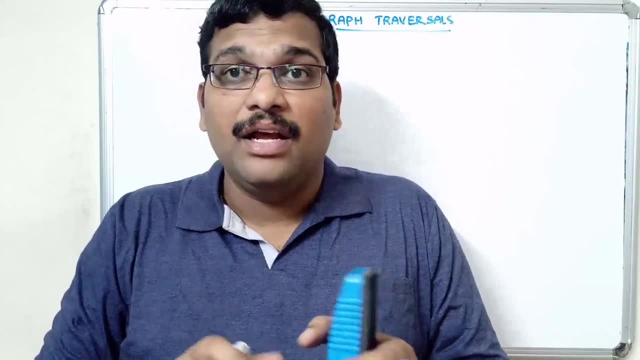 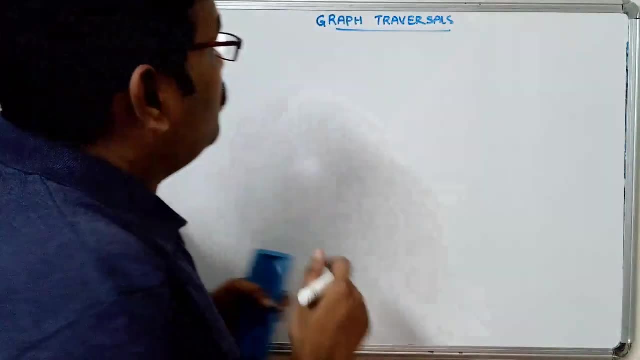 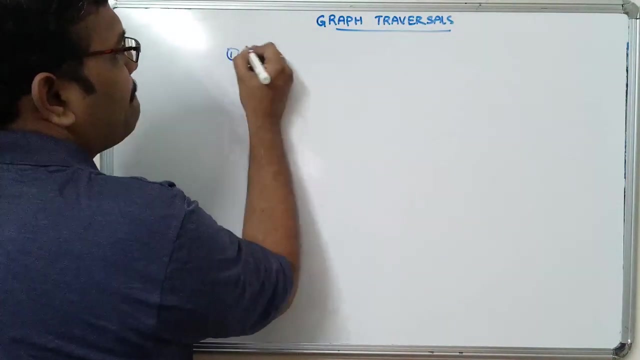 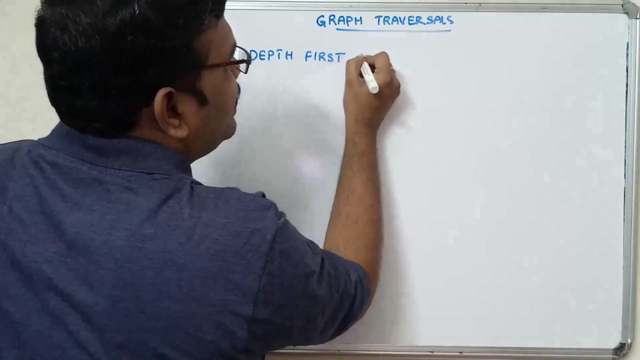 the nodes without any repetition. That means every node of a graph should be visited only once. Now we're having two types of techniques in this: graph traversals. So the first one is depth first search traversals. So what does it Foreign Web Reference come in here? 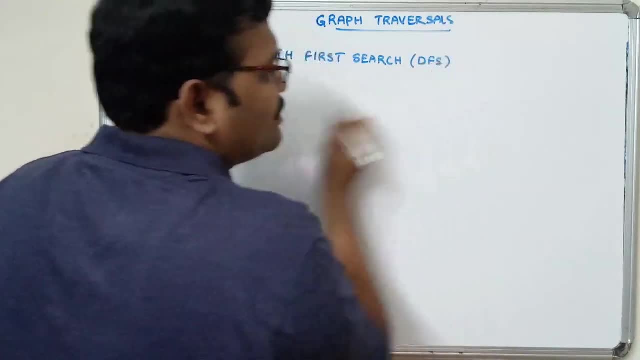 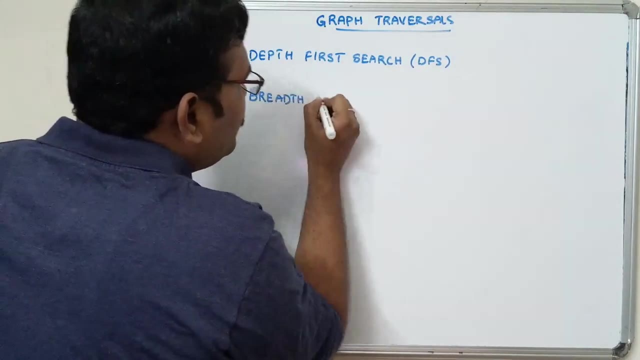 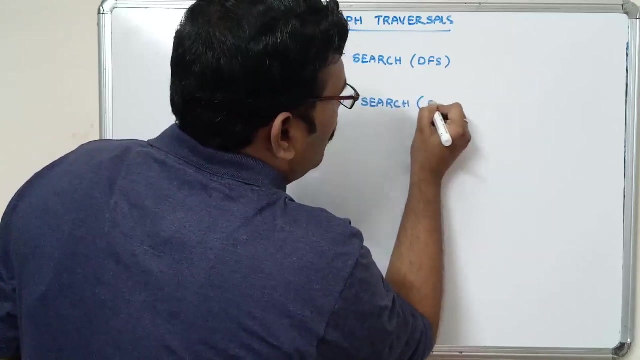 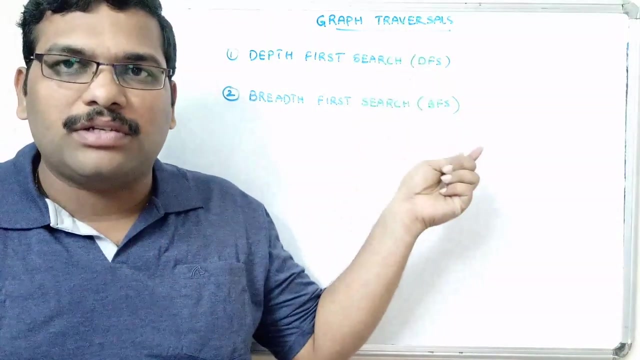 So a truly basic cell, it is called as DFS. and the second one is breadth. first search, which is called a BFS. right, so, based upon the depth, will travel all the nodes of a graph. that is called a DFS. based upon the breadth, that means level. so we have to 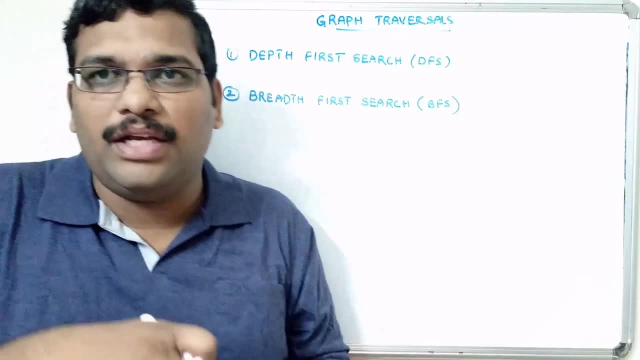 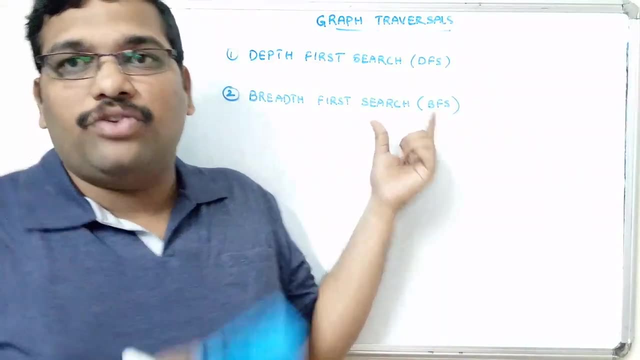 visit all the nodes of a same level, then only we will shift to the next level, so that in such a way, we will go with the BFS, we will implement this BFS. so, in order to implement this DFS and BFS, we will use the stack data structure for. 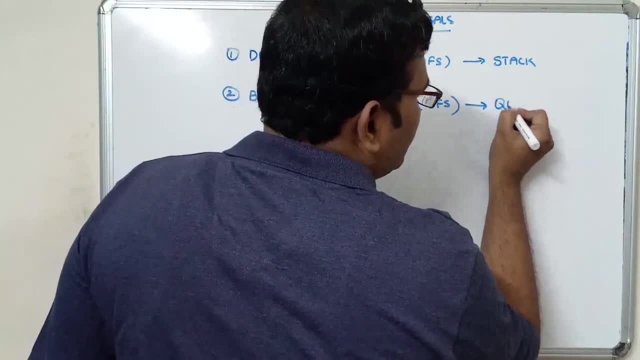 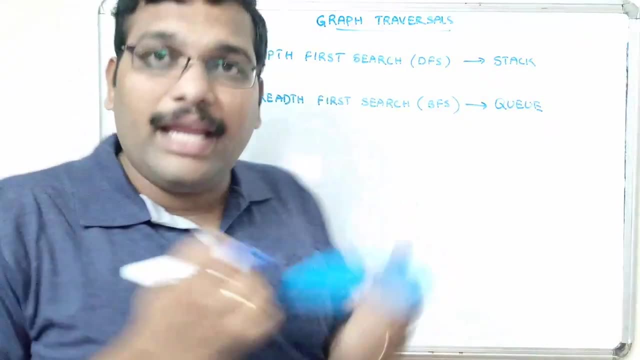 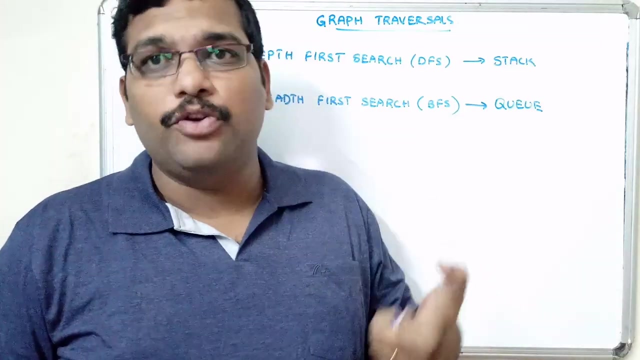 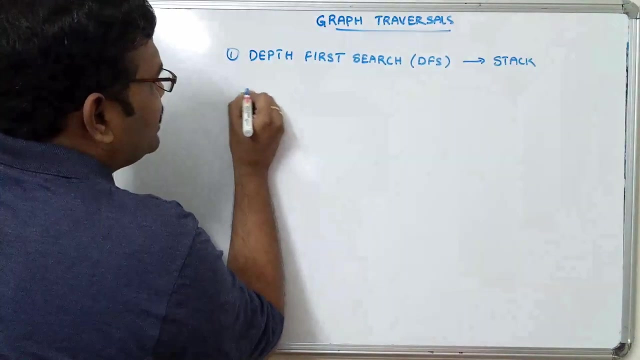 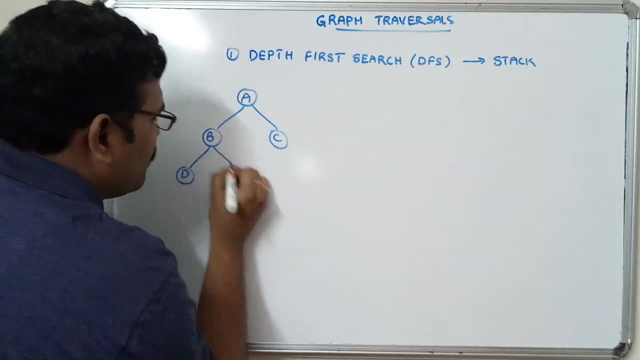 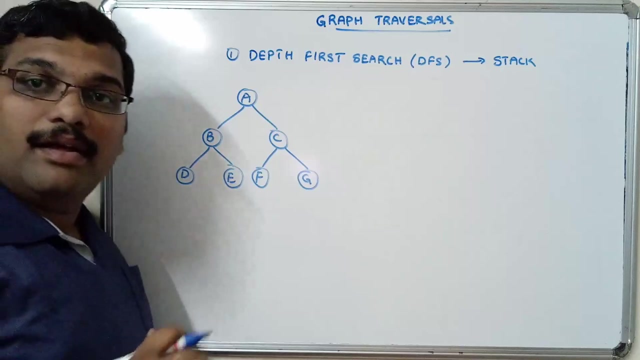 implementing the DFS. we will use queue data structure for implementing the BFS. right so now let us take an example and we will see the procedure: how the DFS will work and how the BFS will work. it is a very simple topic right now, coming to this DFS, see, let us take an example here: A, B, C, yes, so you can go. 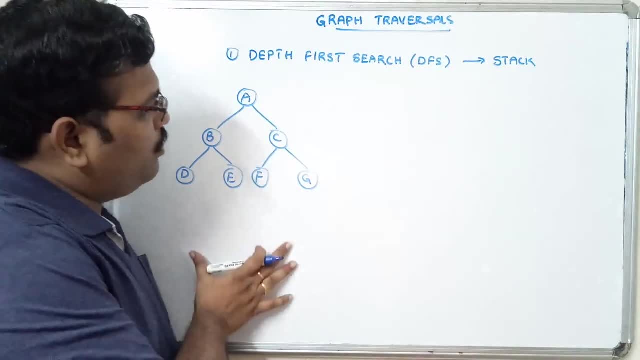 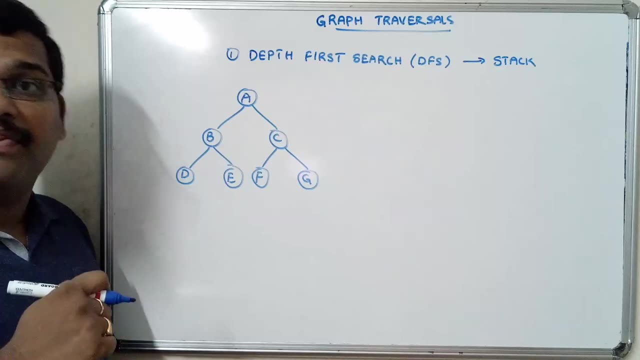 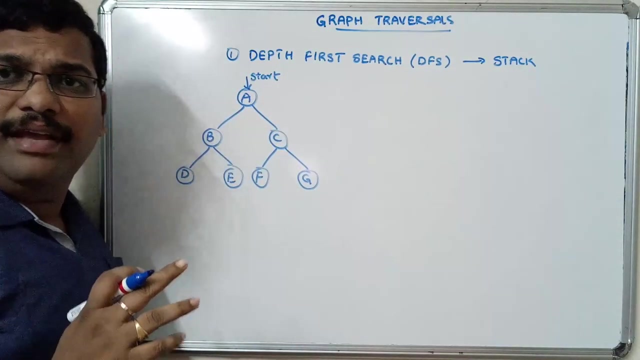 with this one. okay, so you can go with this one. this is a graph, so graph is also similar to a tree, but a graph can contain cycles. that means loops, so this is a graph, of course. so now, first, let us assume this one is a start, so we can assume anything. any node can be a. 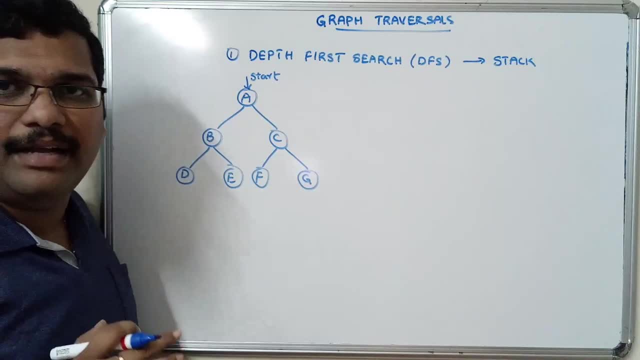 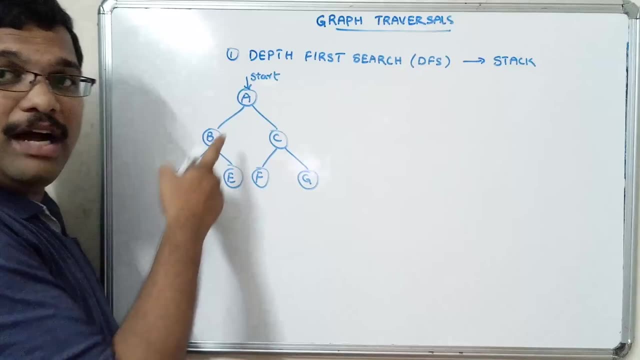 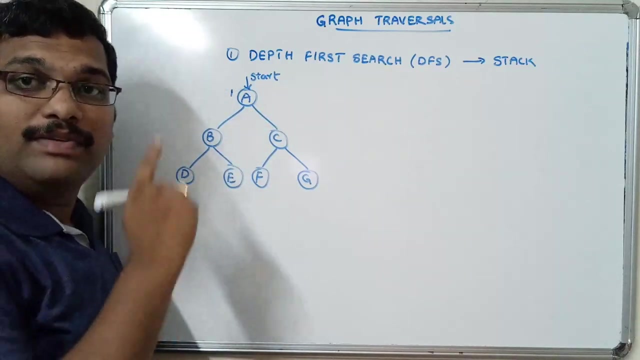 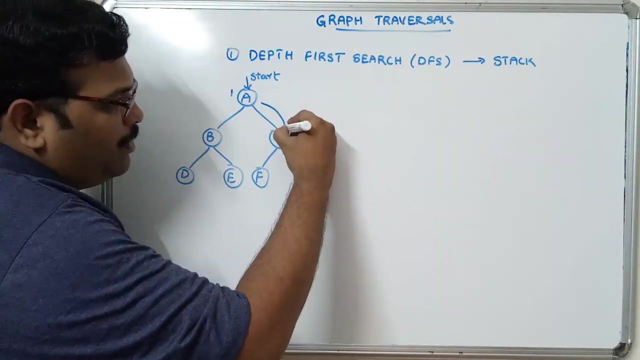 start. okay, I will assume that a start for simple understanding. so I will visit one by one. okay, after visiting this one, after visiting this one. so I will place a weight as one. I have visited a. I have placed it as one. now I am coming to C, right, so you can go. 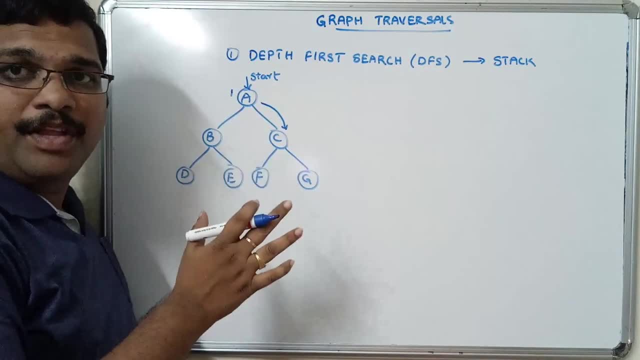 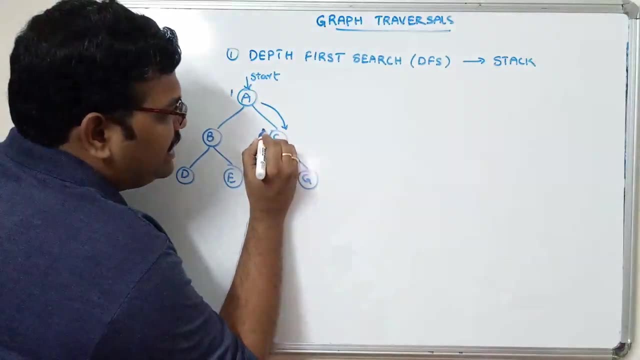 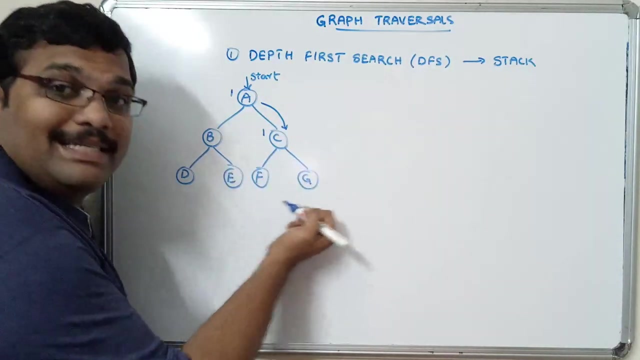 with the B or C. anything else? okay, both are same. you can visit either B or C so we can get a different outputs. okay. so I will visit C, so the C weight is one now from the C again, there are two adjacent nodes so we can visit any one node, okay. 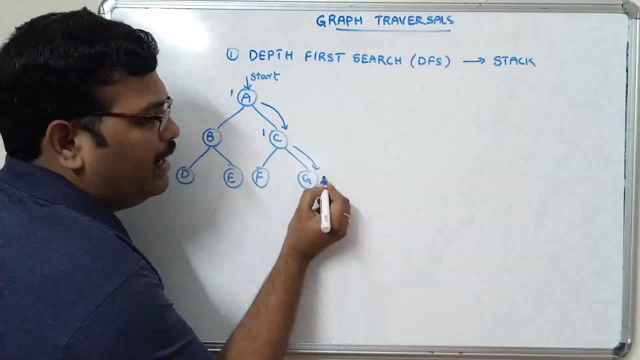 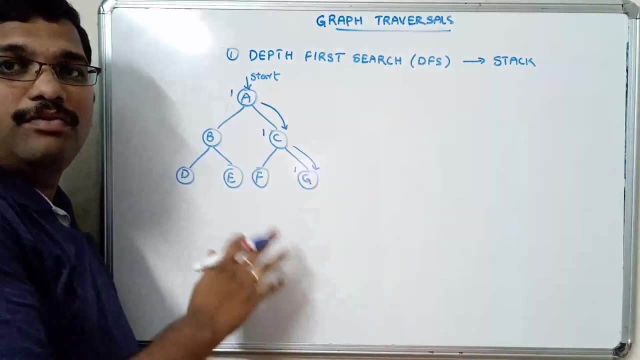 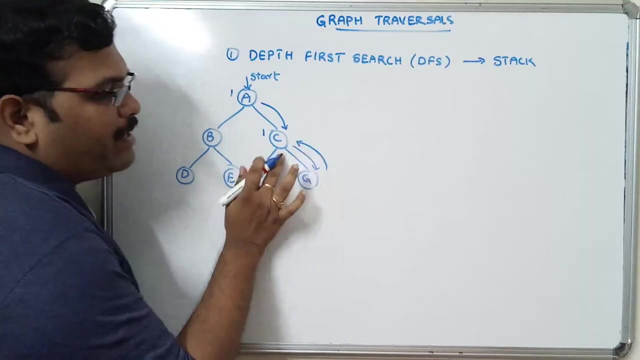 so I will go with the G and the weight of G is one. now, it is a leaf node, there are no nodes. okay, there are no adjacent nodes. we should not say it is a leaf node, we are not having any adjacent nodes, so backtrack, backtrack C and go with the another adjacent node. 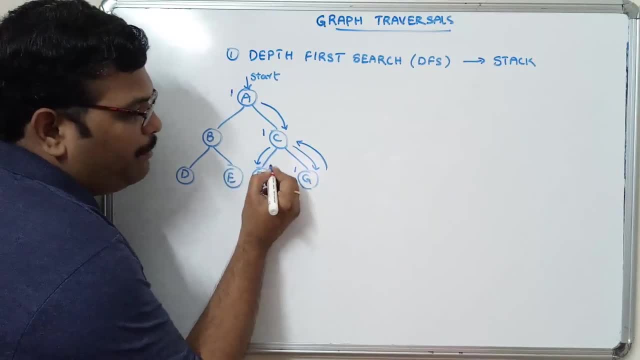 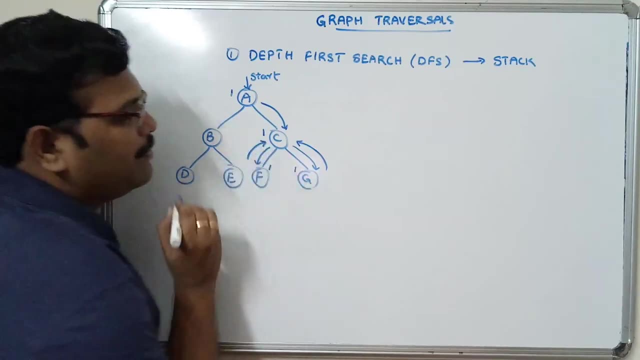 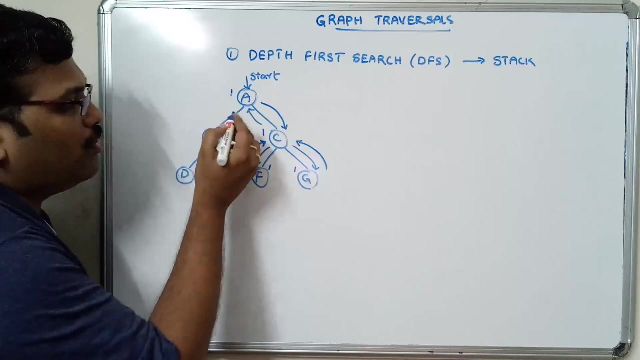 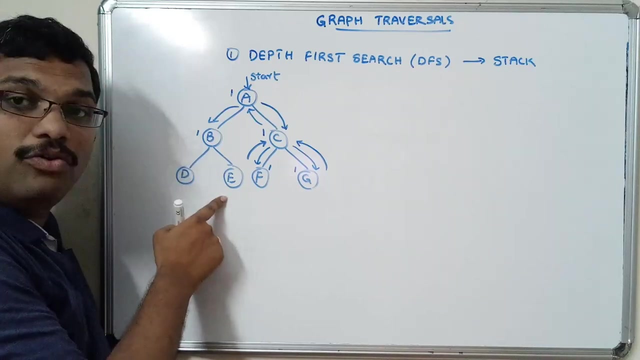 rut and mark it as one. so here also there is no adjacent nodes. again backtrack, again backtrack. so again the node is visited, so go with the adjacent node. so B will be one. now again B is having two adjacent nodes. we can go with the dev in the backtrack C, so go with the. 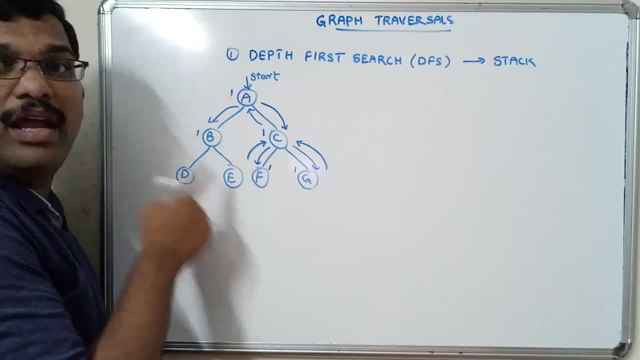 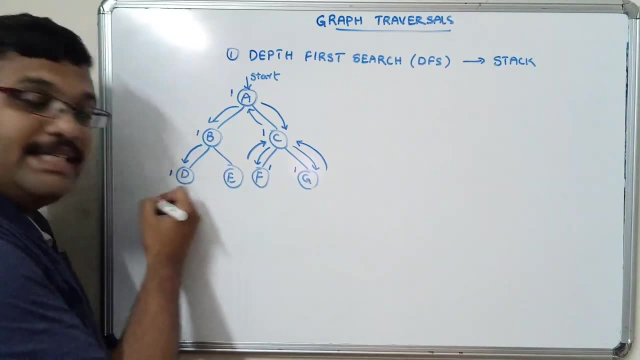 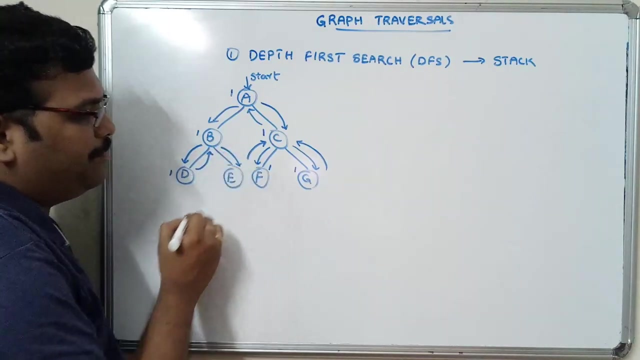 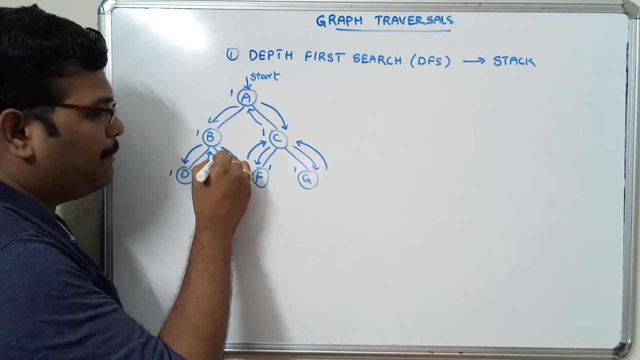 D or E, anything, okay, so I will go with the D mark as D1. again, there are no adjacent nodes. backtrack, right again. go with the E and go with the one. so there is no nodes. okay, there are no adjacent nodes. backtrack and again, backtrack again. we came to the start node and there are. 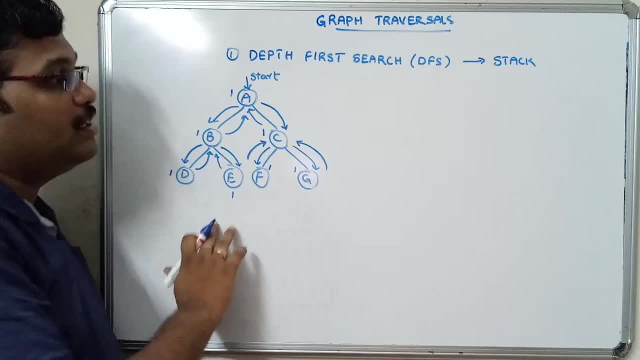 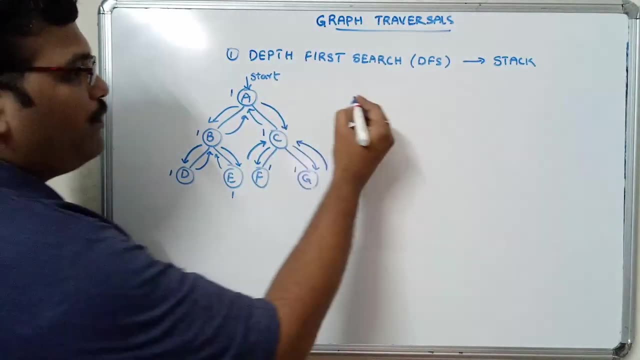 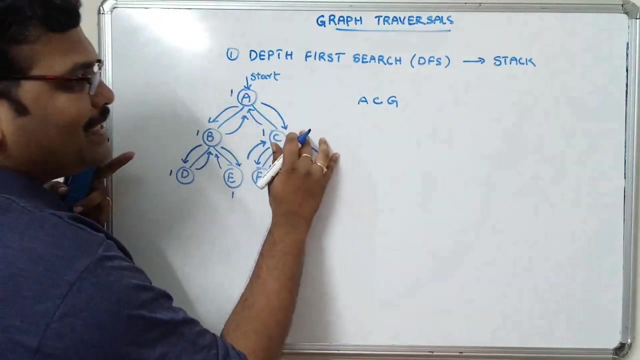 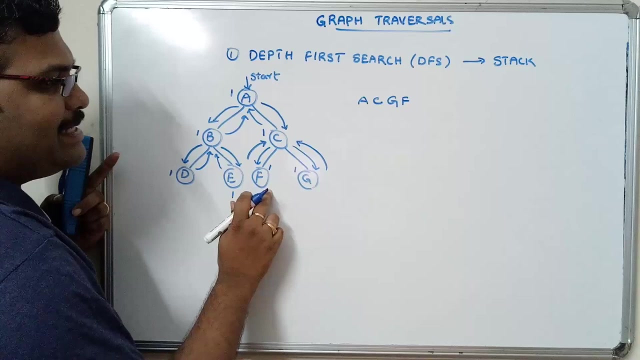 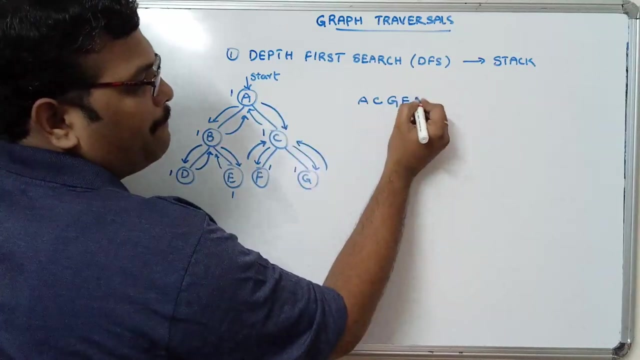 no adjacent nodes. there are no adjacent nodes. so this is how we can use this DFS. so first we have visited A, then C, then G, again backtrack C. so already C is visited. so we should not write C, next F, D, right next no adjacent nodes. again C. C is visited, again A, A is visited, B, B, and then we. 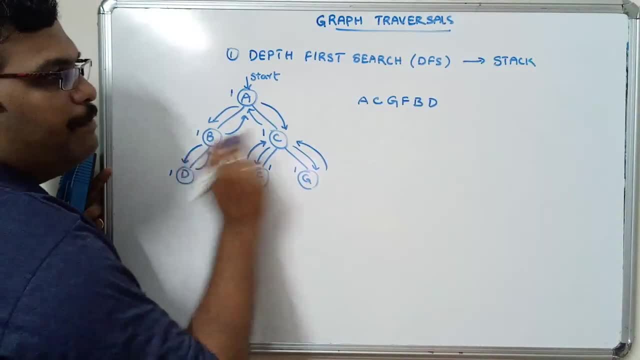 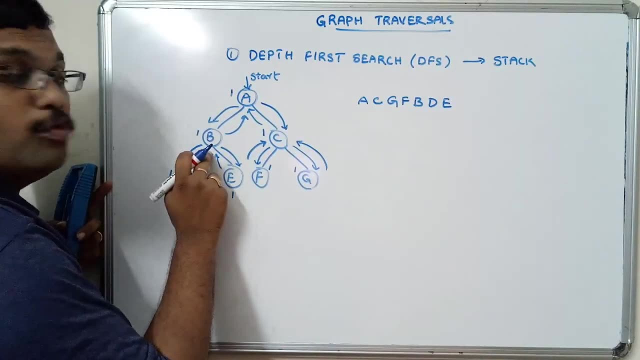 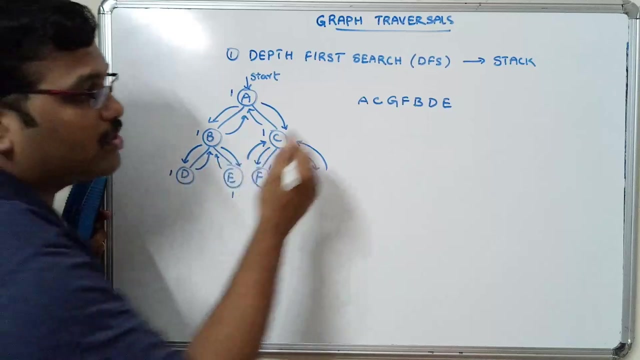 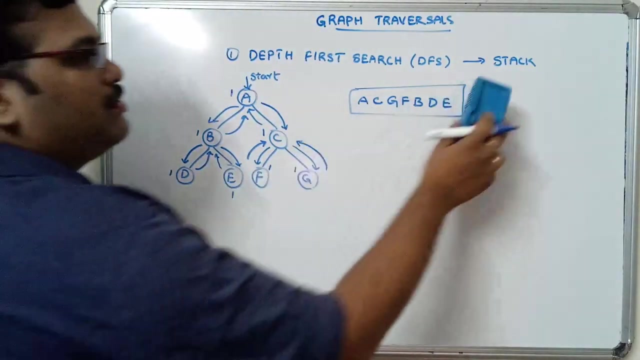 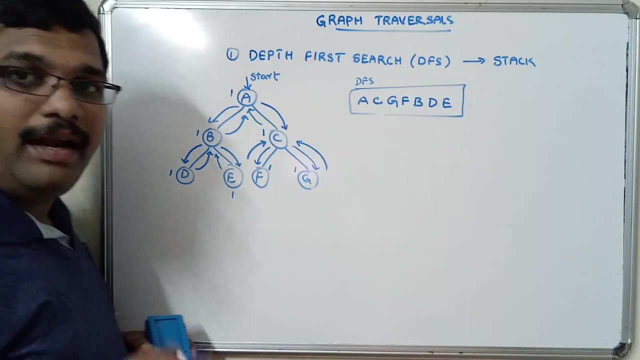 have visited B: no adjacent nodes. backtrack B already there. no E. so E, there are no adjacent nodes. again, backtrack to B. B is there. backtrack to A: A is there. so there are no adjacent nodes, any other adjacent nodes? so so, so, so, so, so. so this is the DFS of a given right here. so this is the DFS for the given graph right. 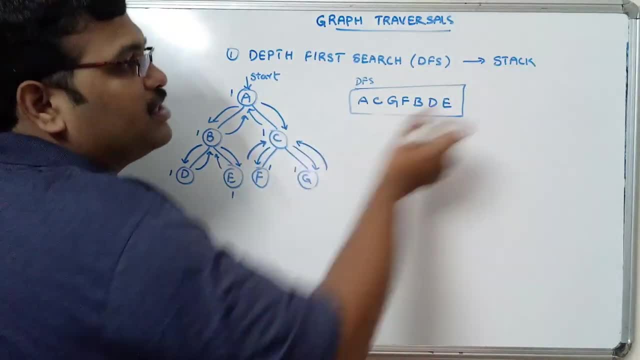 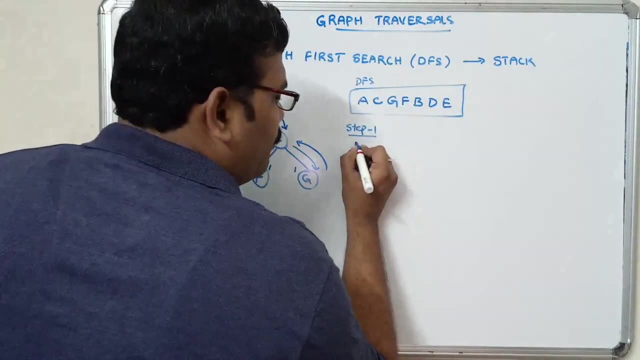 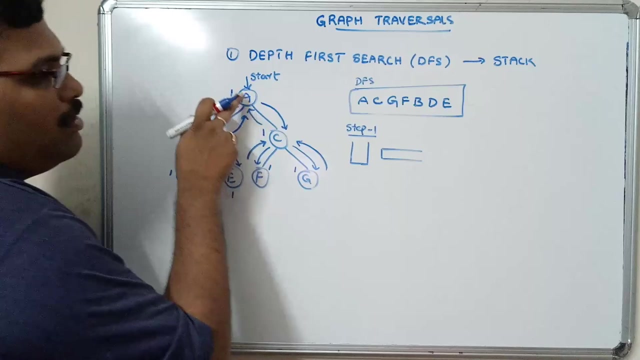 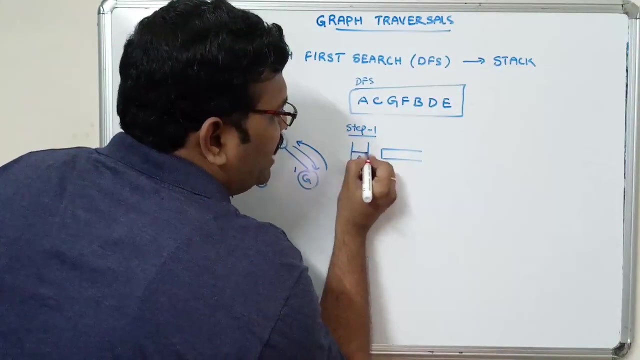 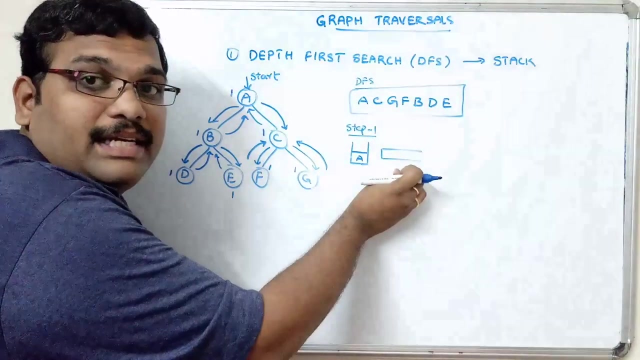 now we go with the implementation part. so for implementing this one we will use the stack. so for the step one, for the step one, consider a stack and consider the DFS expression. right, so starting node, push the starting node into a stack. so A will be presented here. so A is pushed here. now pop the A and placed it. 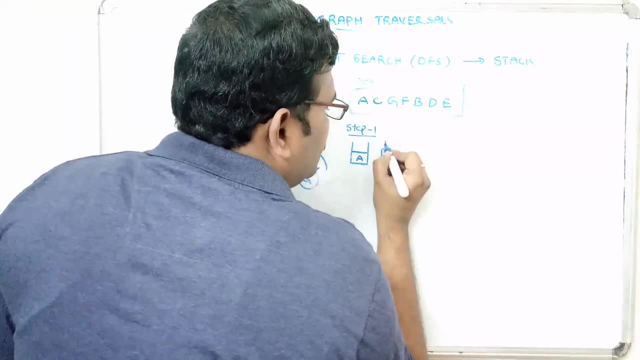 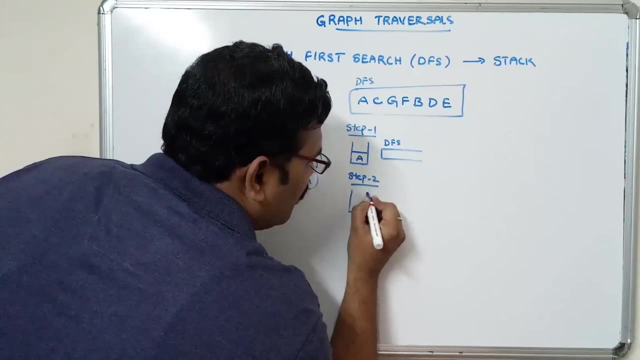 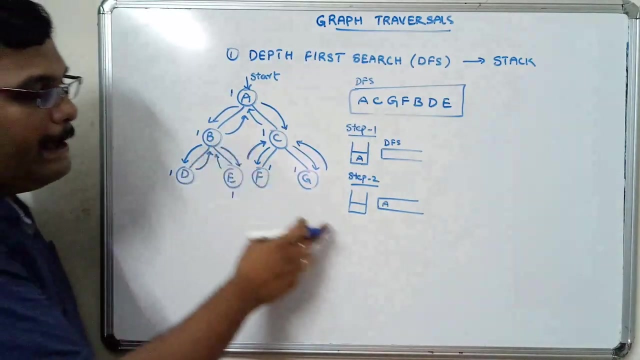 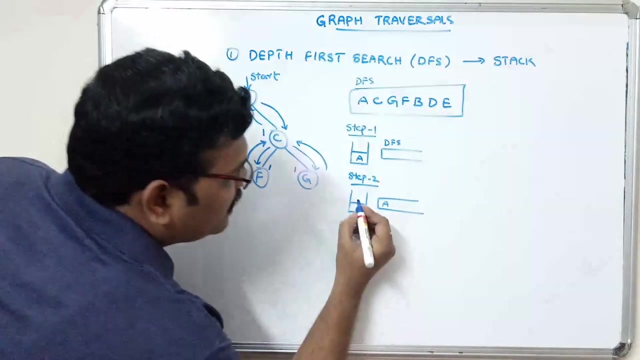 in the DFS expression. right? so this is the DFS expression. so step 2. you know step 2. so popping A and placing A here. now place the adjacent nodes, place the adjacent nodes here. so we'll go with adjacent nodes B, C. push the adjacent nodes of A, push the. 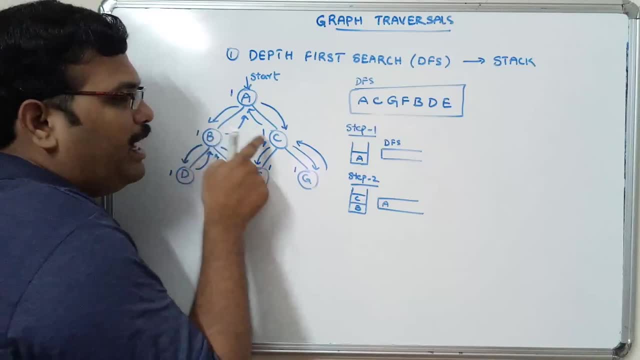 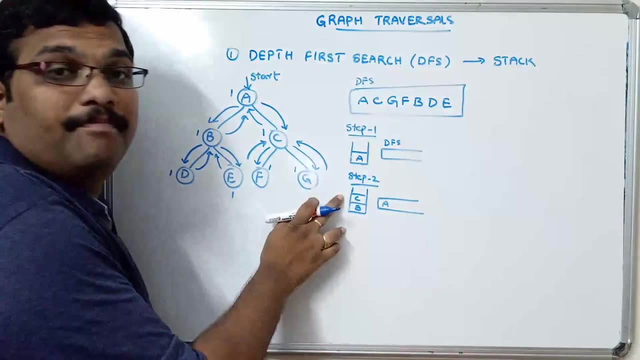 adjacent nodes of A. so what are the adjacent nodes of A, B and C? so we can write B first, we can push the B and then C, or we can push C and B. so if you push the C and B, the output will be different. so both are same. so here, both. 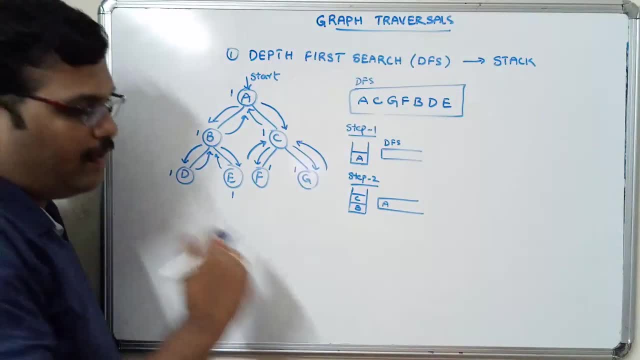 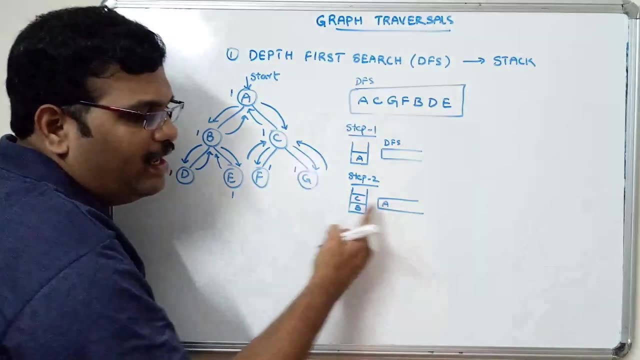 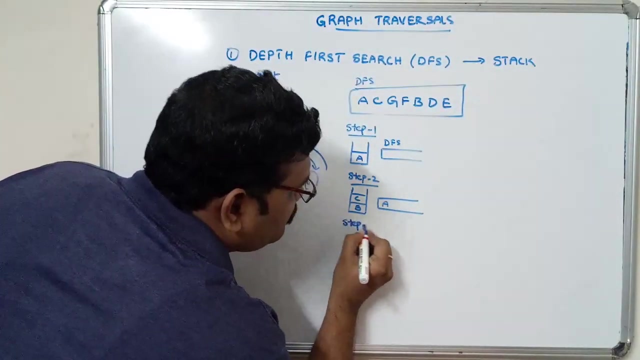 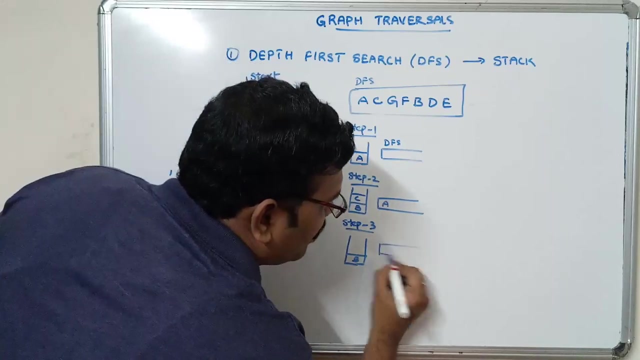 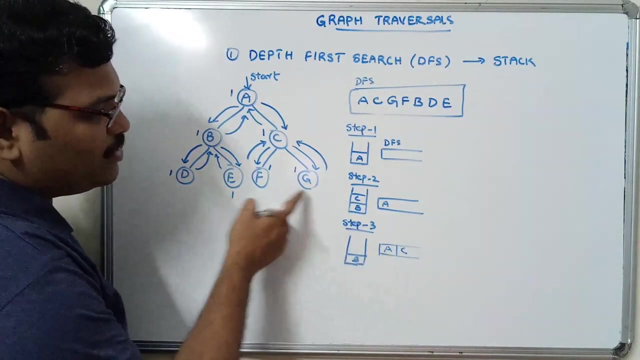 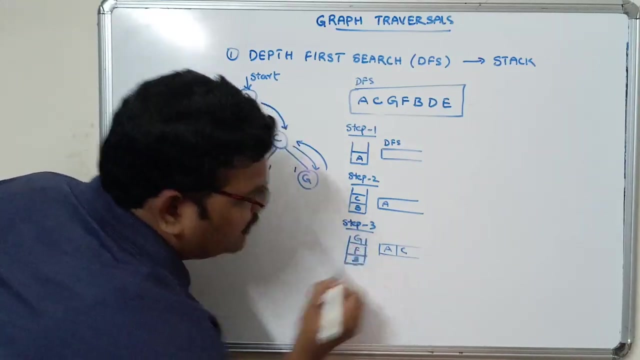 are the adjacent nodes. we can visit any node, right. so next step: we have to pop the. so already C is visited, so we have to pop the C and push the adjacent nodes of C on to the stack. so step 3: B, A and C. A and C. now what are the adjacent of C, F and G? so F and G, right. 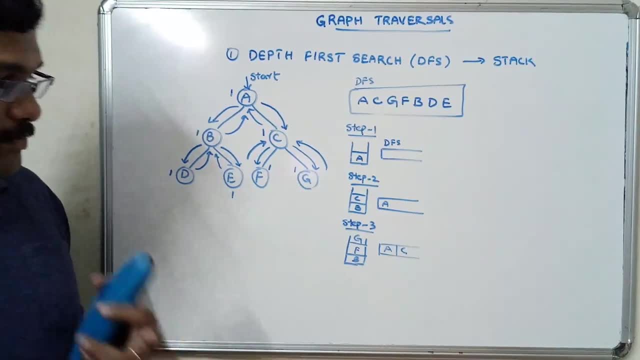 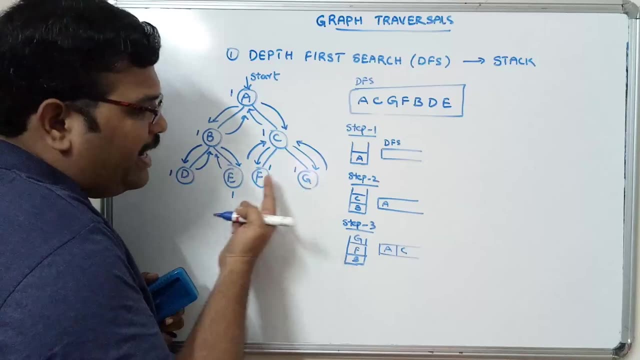 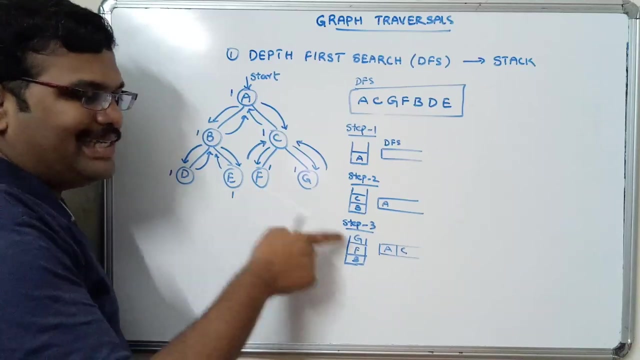 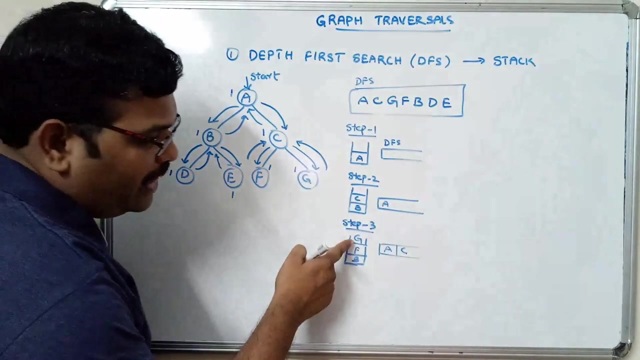 B, F and G. so we can write first, we can push first F and then G, or we can push first G and then F. anything is correct, okay, so, and pushing up yes first and G in the next. now remove the element and push the adjacent nodes of that node. so here G is a leaf node, right? so it doesn't have any. 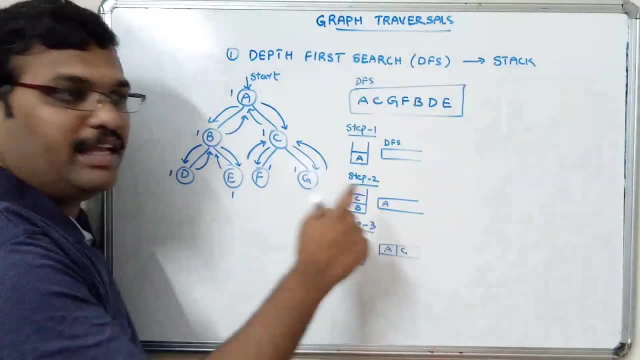 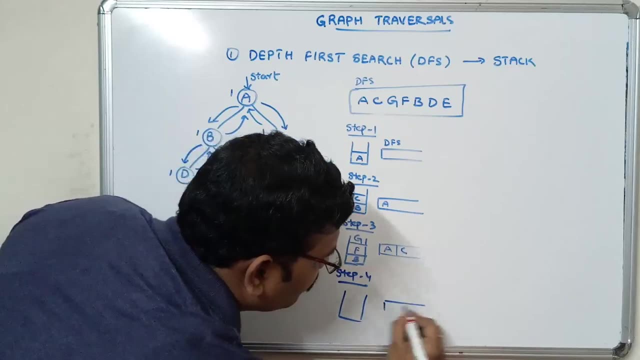 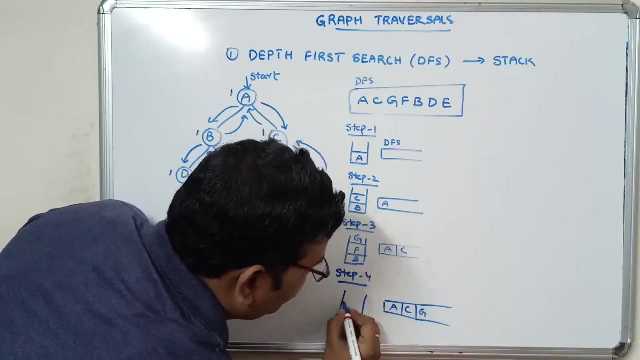 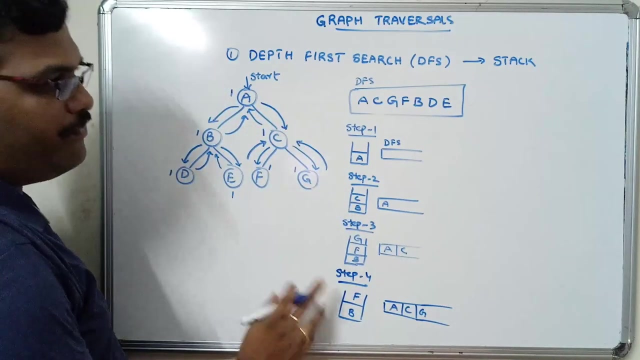 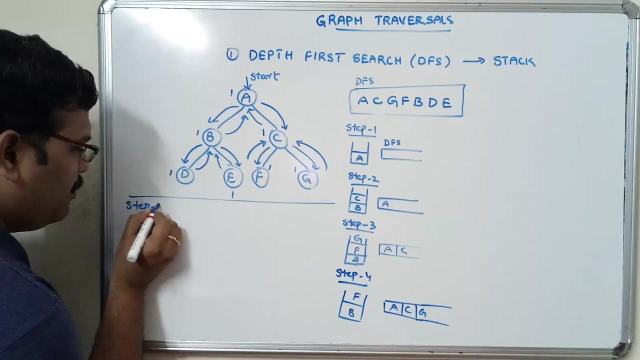 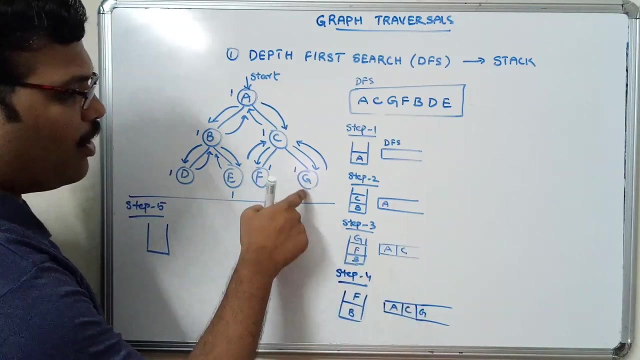 adjacent nodes. so just pop that node and place in the BFS. so step 4: A, C, G and G. so B and F. are there B and F? mine the yön öf A, C, G. okay, then step 5 say so here G is not having any deserve notes. leave it. 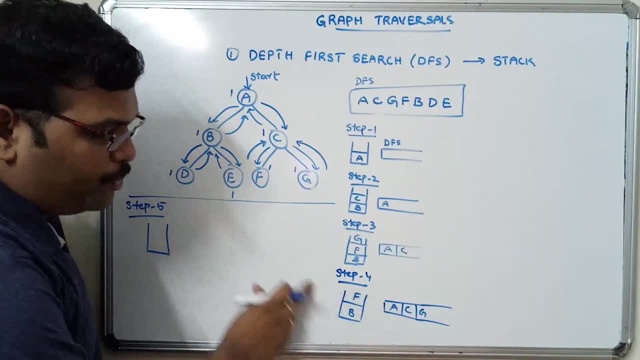 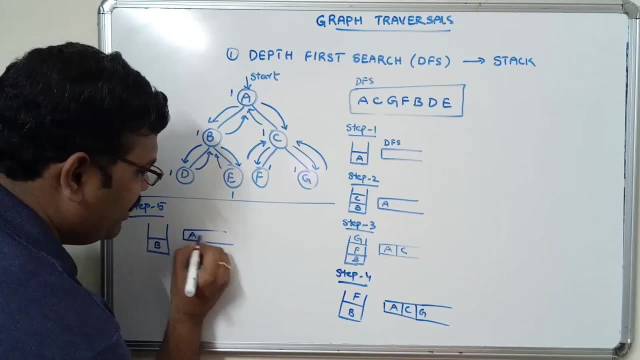 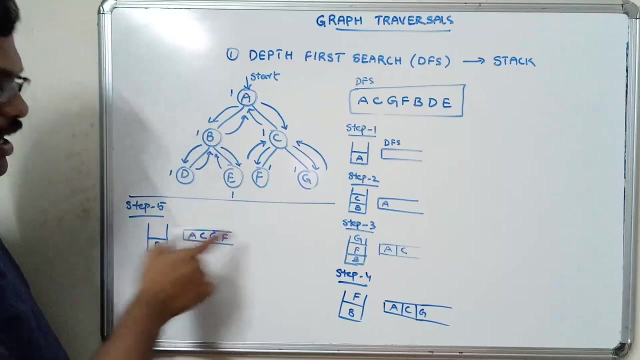 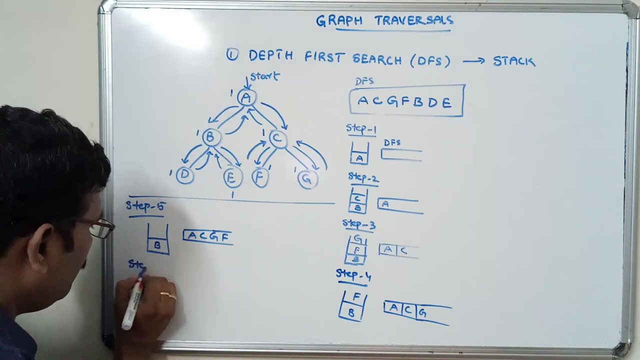 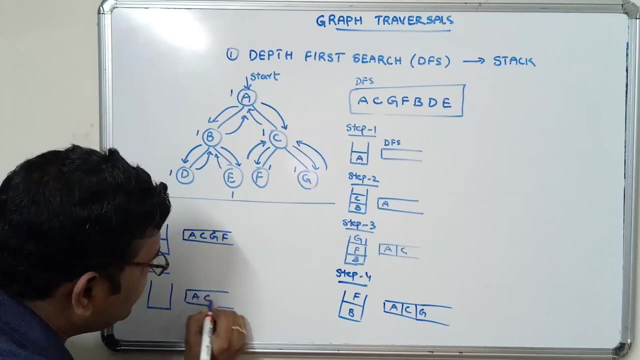 now: yep, remove the F and push all the edges and de sünkün. so already the BFS expression is having A, C, G, and now we are placing F, F here. so F is also having no adjacent nodes. leave it now. B step 6 stack is empty. A, C, G, F and B. 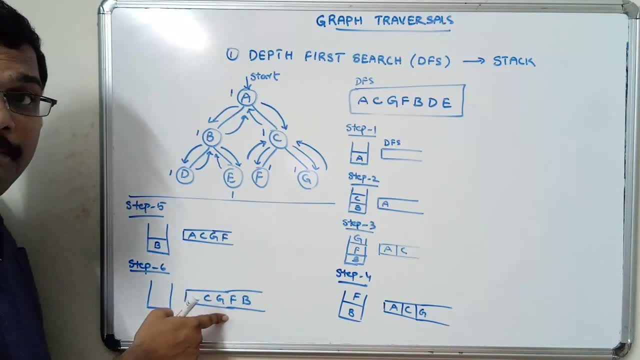 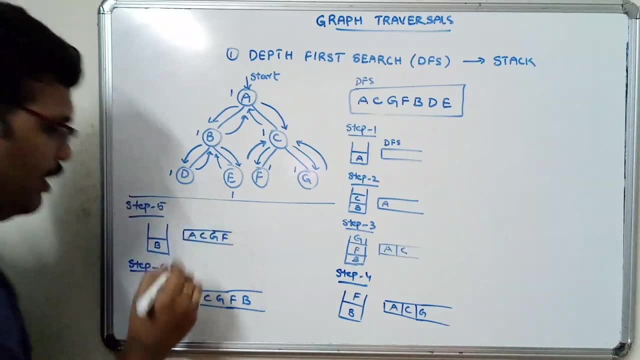 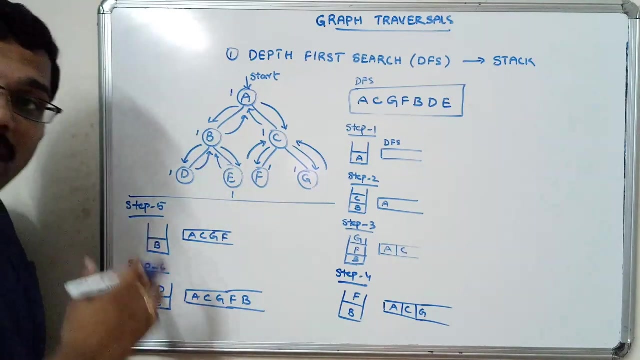 so just pop the element and push the adjacent nodes of that element. so what are the adjacent nodes of B? that are D and E. so first I will push E and then B. so anything we can do, first D and then E or first E and D, because both are the adjacent nodes. 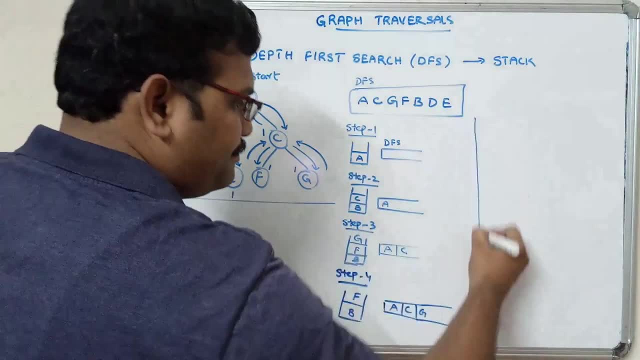 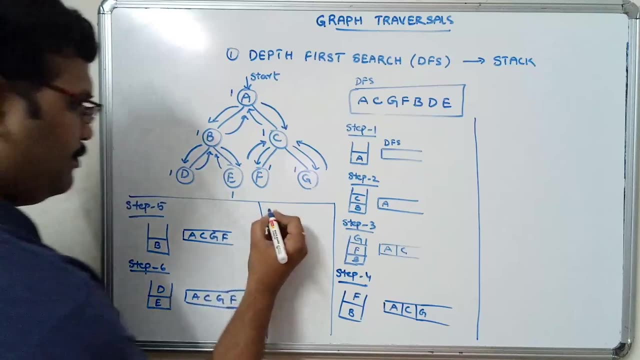 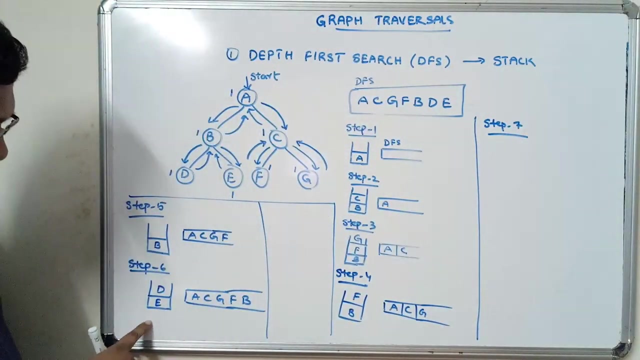 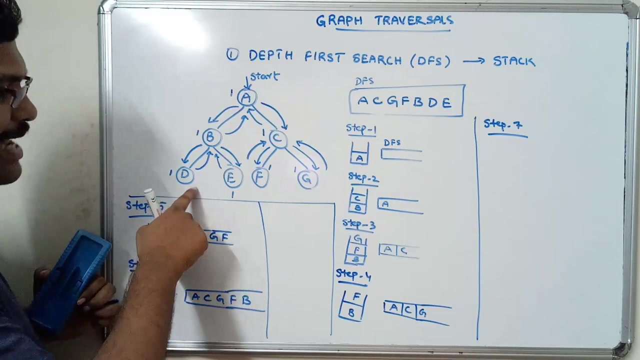 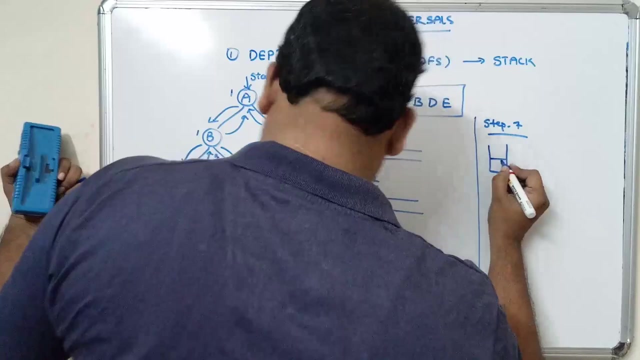 so after that, after that step 6, now step 7, what we have to do again pop the element and push the adjacent nodes into the stack. so here D is having no adjacent nodes, just pop the element. so step 7,, E and in the BFS. 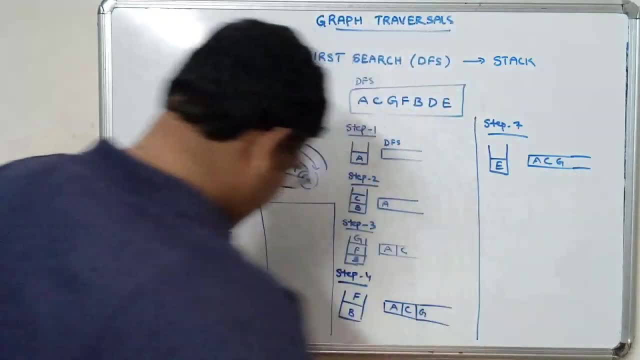 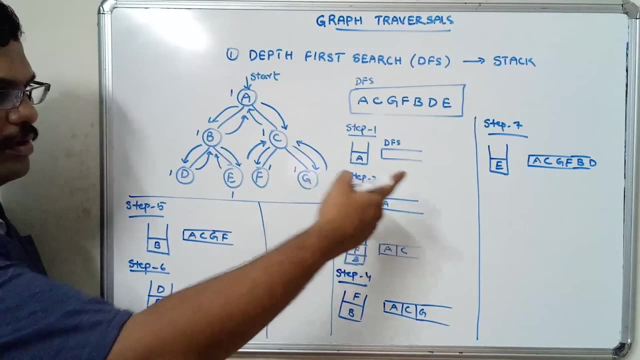 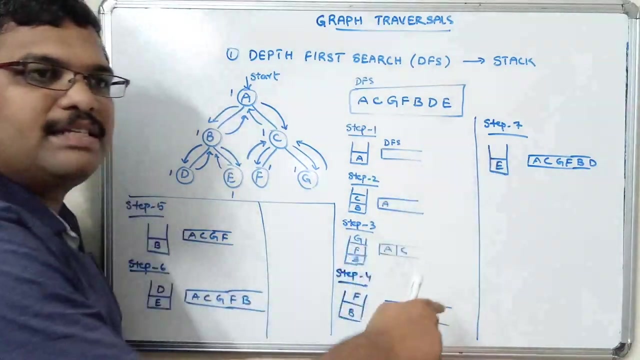 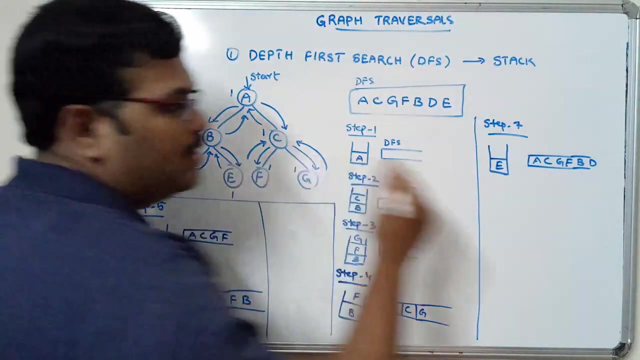 A, C, G, yeah, D and F, B and D. right now, only one element in the stack. the same thing. apply the same thing: pop the element from the stack and place the adjacent nodes of that node into the stack. here E is also having no adjacent nodes. 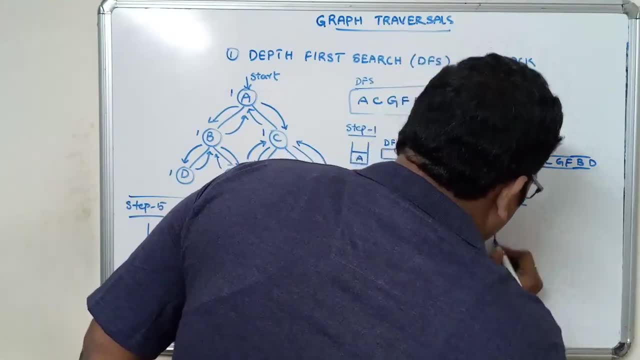 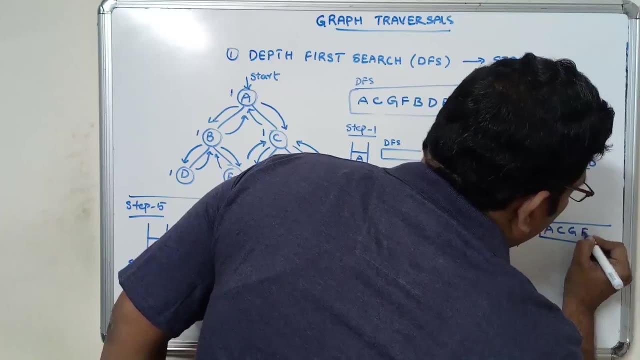 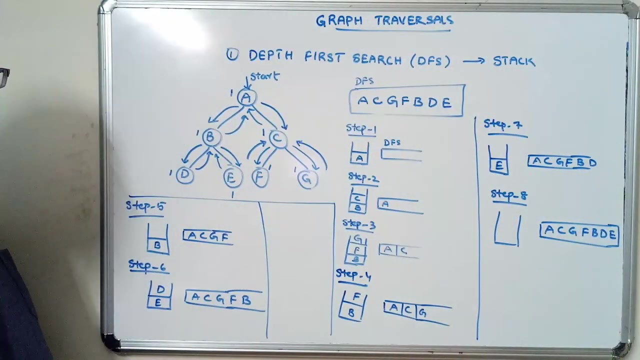 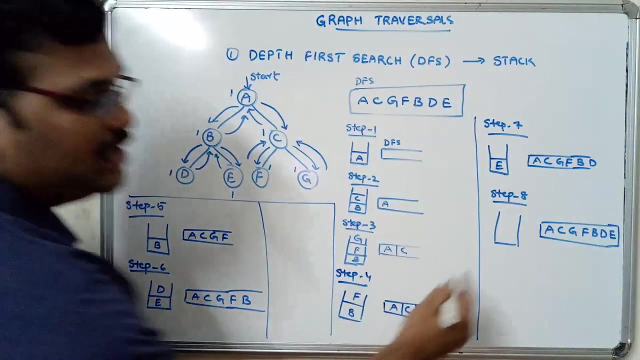 so just after step 8, the stack is empty and the DFS traversalen is B, D and E, right. so stack is empty. stack is empty, right. so don't get confused. just I have written empty, okay. okay, this is empty, stack empty, right. 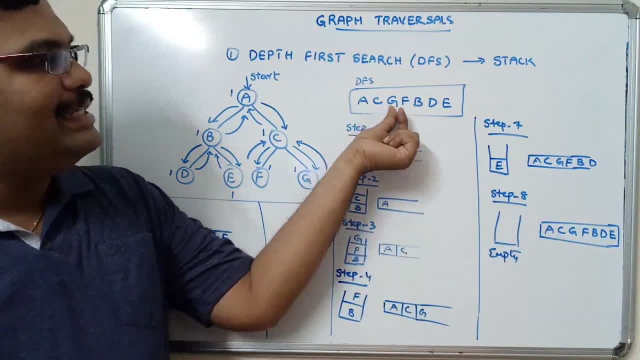 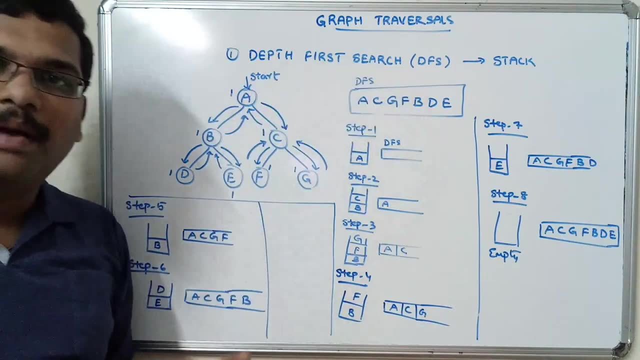 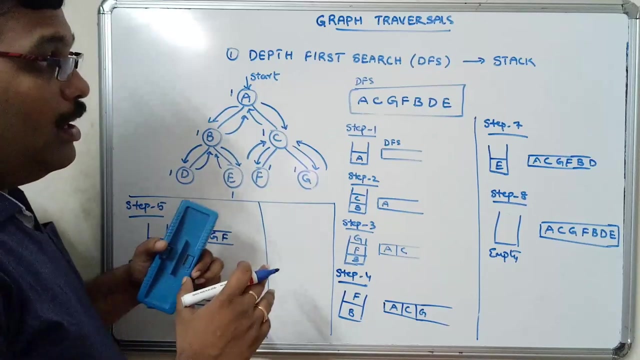 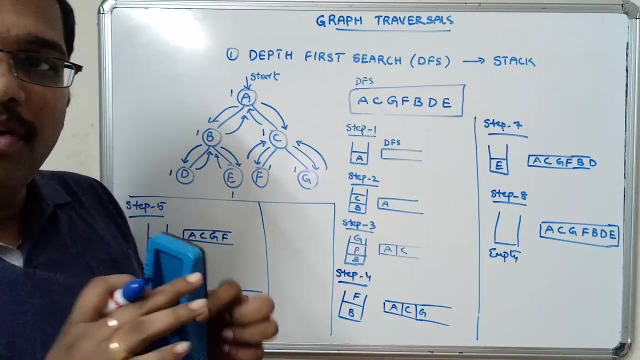 so if you observe this one, we have got the same thing: A, C, FBDE. so by using the stack we can implement this DFS approach right? so this is one way we can implement this one. so one more thing I just want to say here. both are adjacent nodes. need not worry to push the order of. I mean. 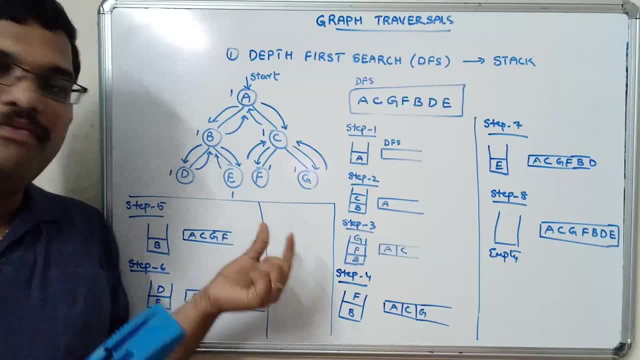 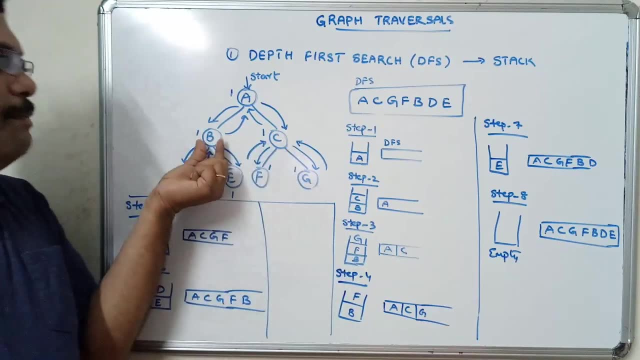 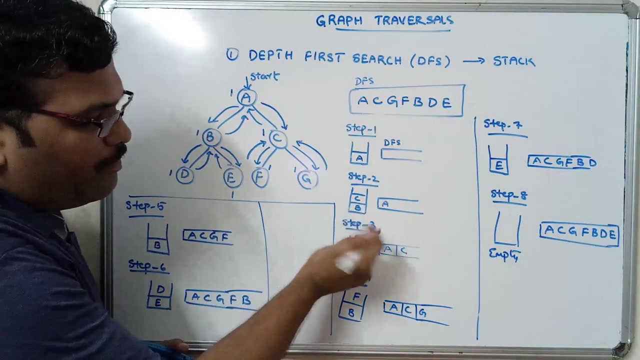 pushing the order of nodes into the stack so we can follow any order. so you can push B first and then C. next we can push first C and then B, so that we'll get a multiple number of outputs. so if you push first to C, so here we have. 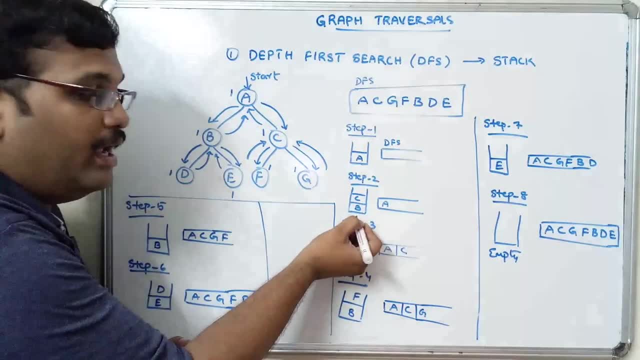 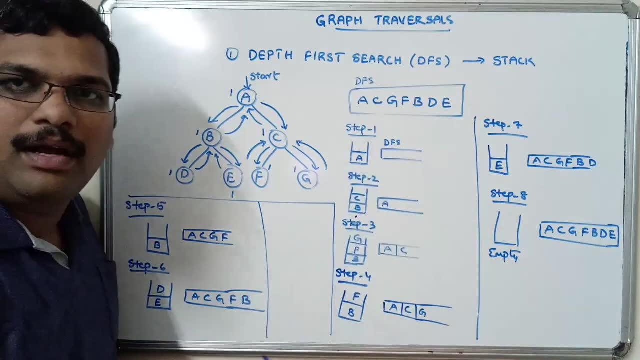 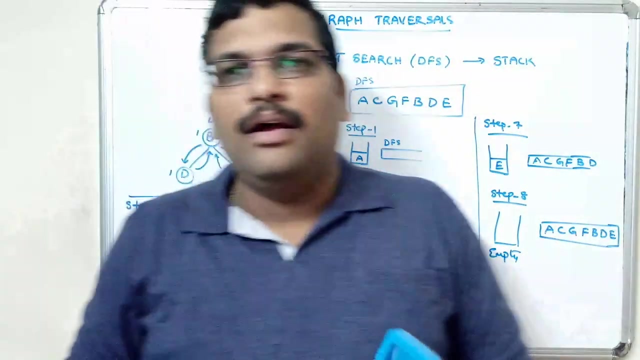 applied, I mean push operation, first on B, then C, so we got this one. if you apply first to C, then B, we'll get the next one, another one, I mean another output, so don't get confused, right. so hope you understood this session. a simple DFS approach: depth first search for implementing this depth first search. 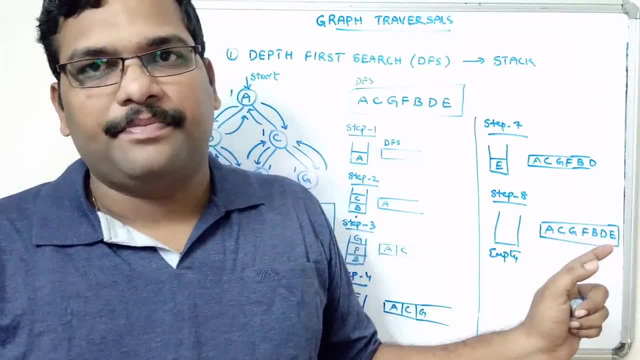 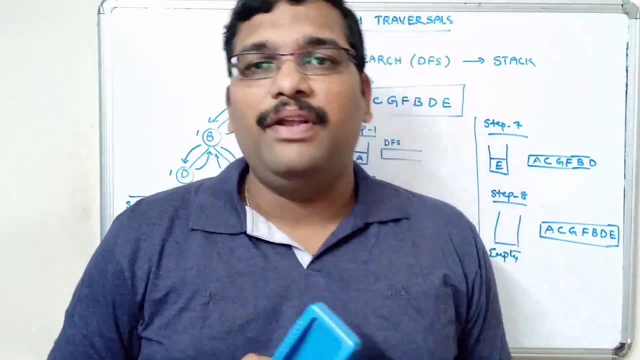 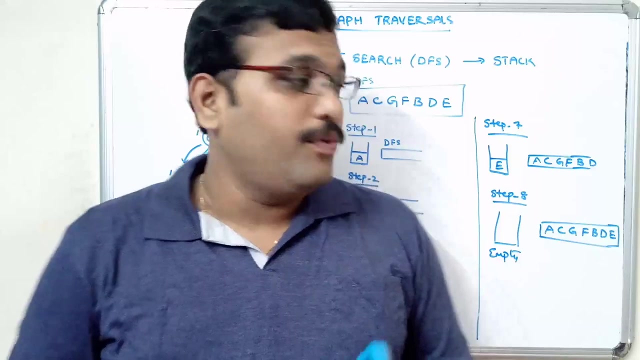 will go with the stack right. so if you have, if you are having any doubts regarding this DFS, feel free to post your doubts in the comment section so that definitely I will try to clarify all your doubts and if you really understood these sessions, like my sessions, you.